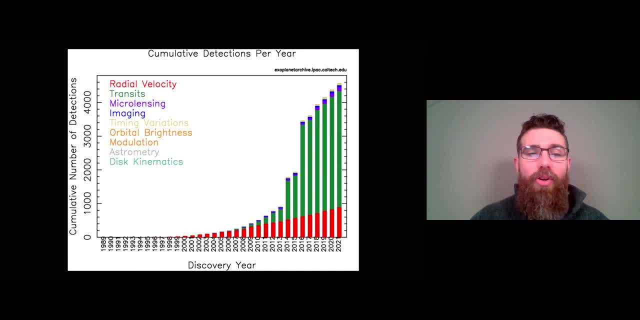 method that they've been detected by- and you can see the majority here has been by the green method, which is the transit method and the one that we're interested in for this particular video. The next most significant one is the radial velocity, which we can cover in a different video. 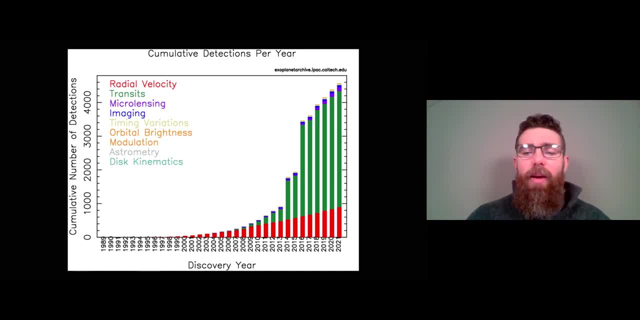 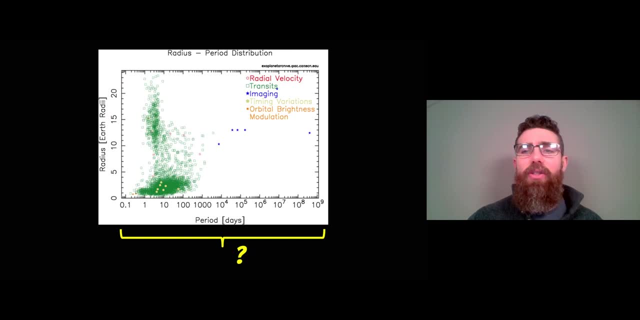 but you can see how there's been a large increase in the recent years. but we've got lots of information about those exoplanets, So how do we actually get them? So if you go on to the exoplanet archive, you can get lots of information. 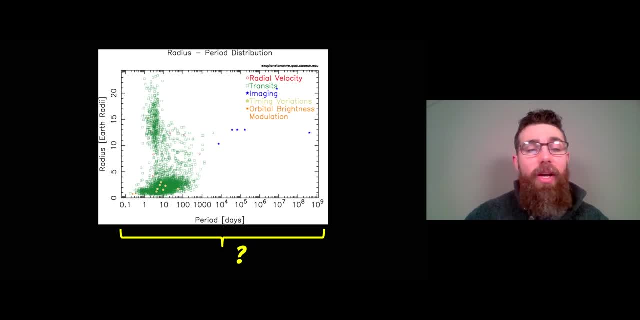 and plots of all of the exoplanets that have been discovered so far. So here is one. We've got the radius of the planet in Earth radii, and we've also got the orbital period along the bottom, the exoplanet. Now, one thing you can see straight away is that the orbital periods are fairly small. 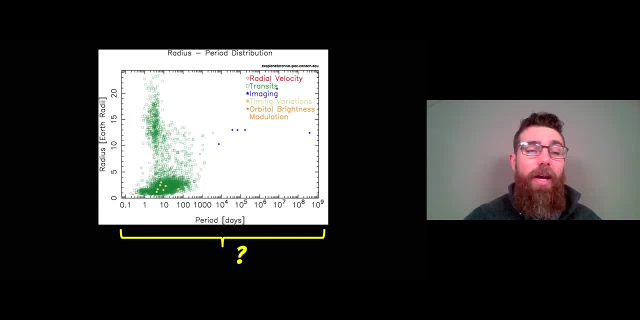 or short, and they're fairly large radiuses when compared to Earth. So we've got a lot of large planets orbiting fairly close to their planet. They're actually easy to detect, which is half the reason, But where do we get that period from? And again, if we were to plot something like the 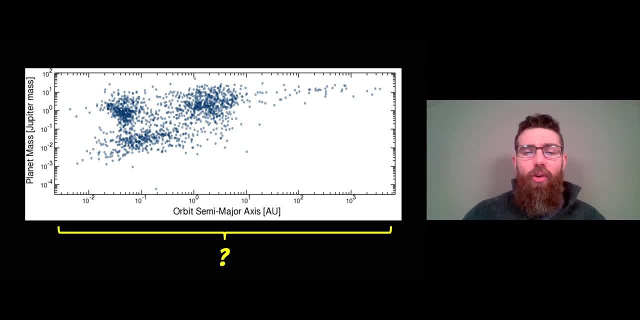 planet mass in Jupiter, masses against the orbit, so major axis along the bottom we can see we've got a distribution here And again it's telling us that a lot of large planets are fairly close to their star, just by the way that there's a bias in the detection method. However, how do we? 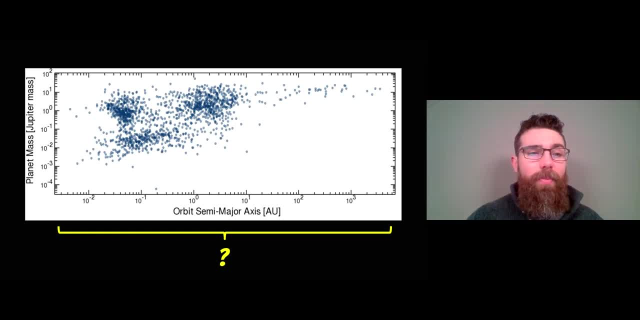 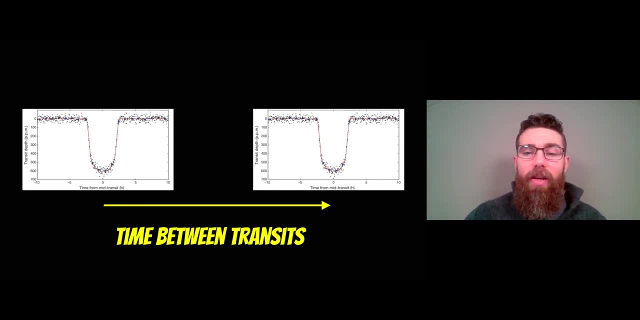 get that semi-major axis which is relating to its orbit. So the easy thing really is the period. So the orbital period we can calculate by measuring the time between the different transits, So as that planet passes in front of the star it blocks out some of the light which you can. 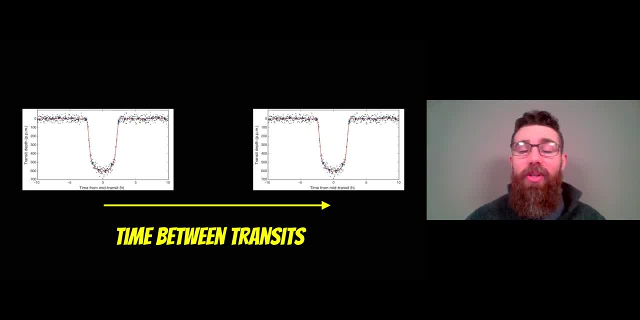 by this U-shaped transit. All we've really got to do is wait for it to come back round again on its orbit and detect the next one. So the time between the transits gives us our orbital period. Now, if you've only got the one transit, it becomes a bit more complicated. 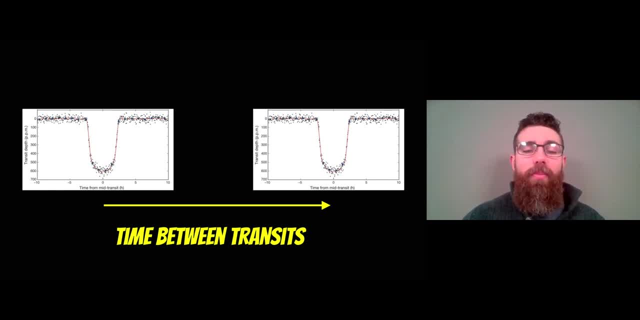 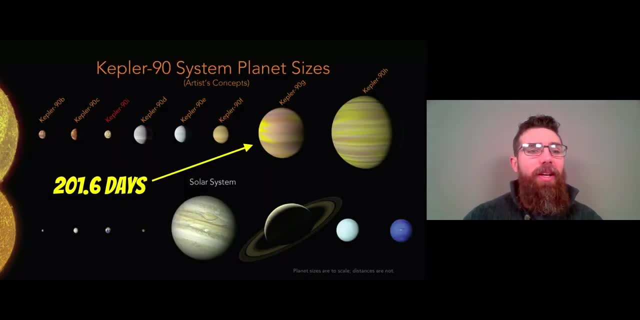 and there are other methods to get the orbital period, But most of the time if we've got multiple transits, we can get the orbital period fairly easily. So let's take an example which we can work towards. So this is the Kepler-90 system and we've got quite a few. 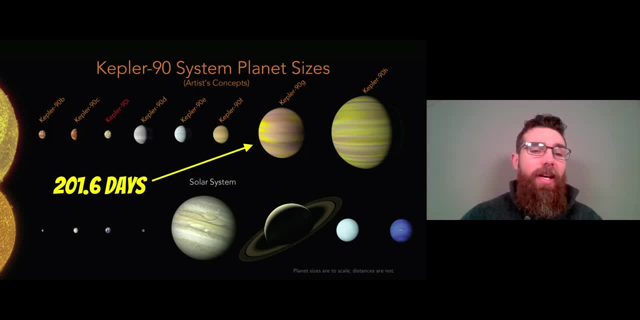 planets here, a large number of planets, And let's have a look at the Kepler-90g, which is a fairly large planet and it has an orbital period of 201.6 days, which has been found by the time between the transits detected. So let's try and find out its orbital, the 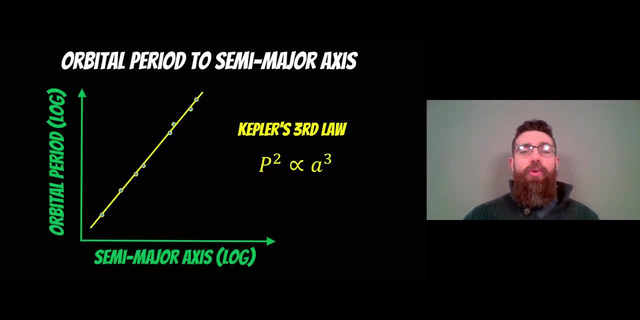 major axis. from that. Now, if we go to Kepler-90g, we can see that the Kepler-90g is a fairly large planet And that's the Kepler-90g in the third law. So that's the Kepler-90g in the third law. So the Kepler-90g in the third law is a fairly large planet and that's the Kepler-90g in the third law. So that's the Kepler-90g in the third law. So if you look at the Kepler-90g, 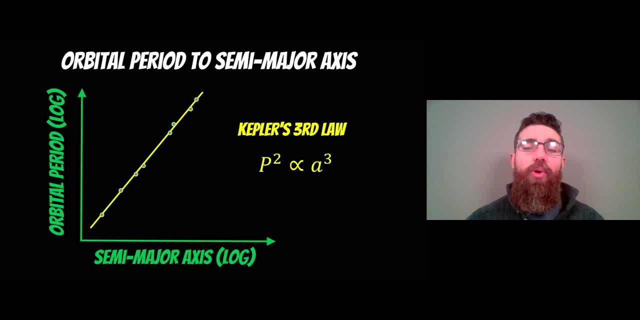 in the third law, the orbital period squared p, is proportional to the seven major axis, which is a cubed. If you create a plot of that, you get this nice straight line when you plot both on the logarithmic scale. So then the orbital period is plotted against. 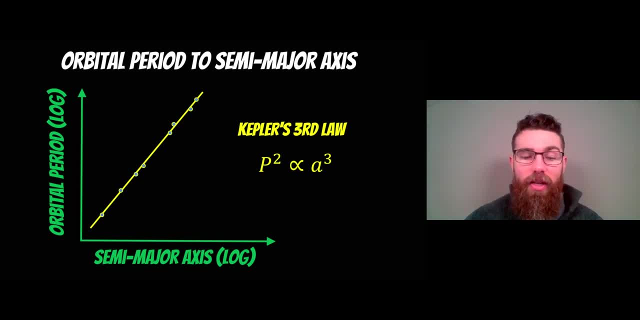 the seven major axis. When it's logarithmic, you get this straight line. Now, this originally came about through the solar system, So the closer planets- so like Mercury Venus, all Mercury Venus all- have shorter orbital periods and they also have smaller semi-major axis. 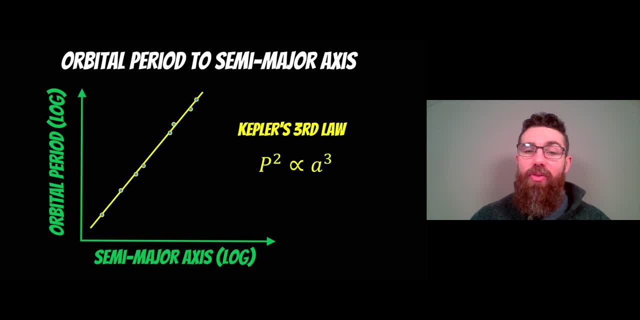 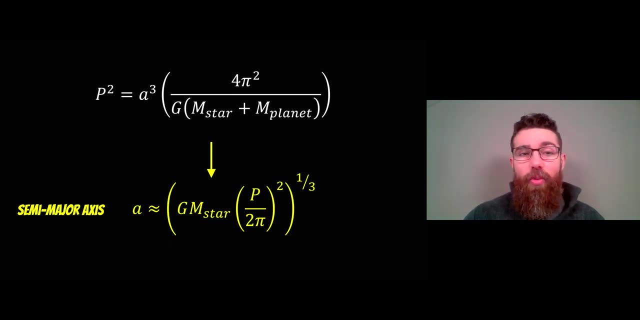 So as you get further out, the orbital period increases and you get this particular relationship. So we can use this to work out the orbital or the semi-major axis. So at the top we have an equation which relates to the square of the orbital period. 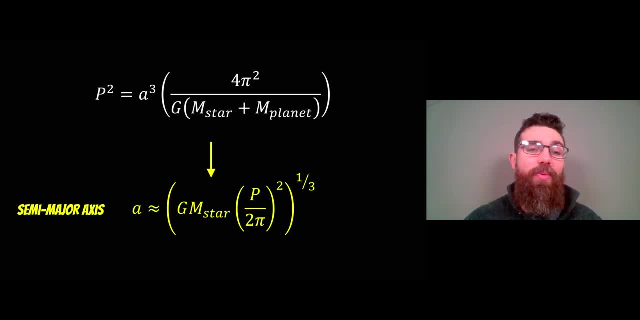 And then, on the right hand side, we have the semi-major axis, which is A. We have also the gravitational constant, the mass of the star, the mass of the planet, And then you've got your four pi squared on the top. 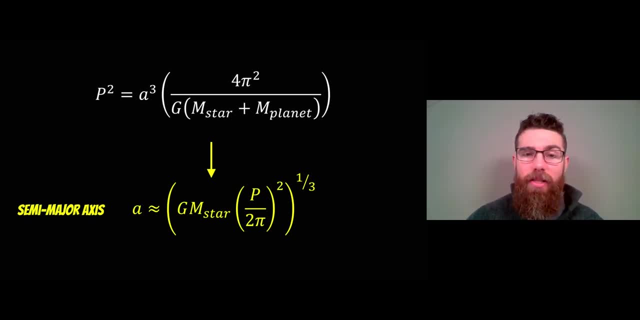 What we can do is rearrange that for the semi-major axis and we get the bottom expression there. Now you'll note that we don't have the mass of the planet there, And most of the time the mass of the planet is so much smaller than the star that it can be neglected. 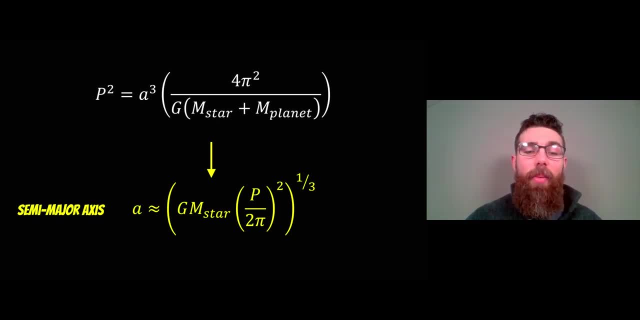 So we're just going to write that. So the approximate semi-major axis is given. So we're just going to write that. So the approximate semi-major axis is given, And the only thing we need in that is the orbital period which we can detect or calculate from the time between the transits.